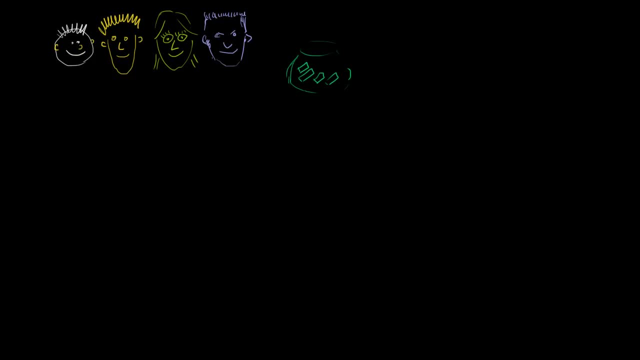 And so they start that process. So let's say that after the first three nights that he the oldest brother here, let's call him Bill- let's say, after three nights Bill has not had to do the dishes. So at that point 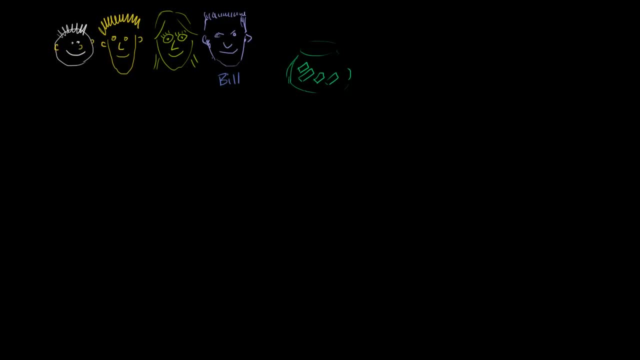 the rest of the siblings are starting to think: maybe, just maybe, something fishy is happening. So what I want to think about is: what is the probability of that happening? What's the probability of three nights in a row? Bill does not get picked, if we assume. 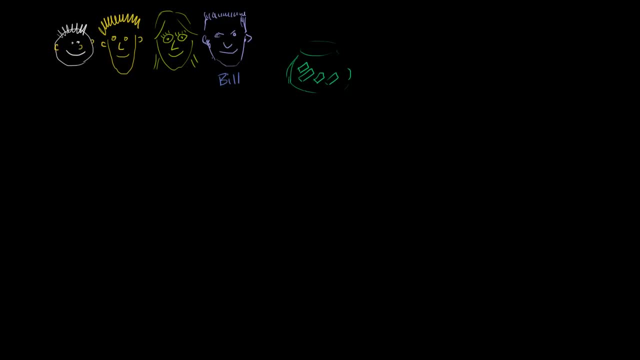 that we were randomly taking. if Bill was truly randomly taking these things out of the bowl and not cheating in some way, What's the probability that that would happen? that three nights in a row Bill would not be picked. I encourage you to pause the video. 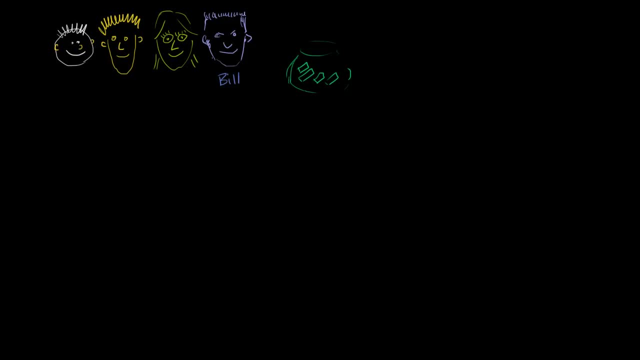 And think about that. Well, let's think about the probability that Bill's not picked on a given night. If it's truly random, so we're going to assume that Bill's not cheating. So assume truly random and that each of the sheets of paper 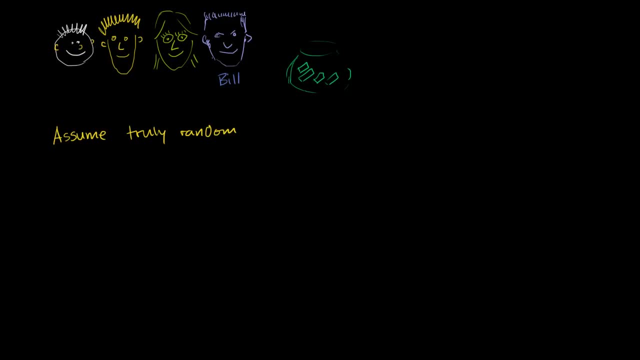 have a one in four chance of being picked. What's the probability that Bill does not get picked? Well, there's. so let me the probability that I guess. let me write this: Bill not picked on a night on a night. 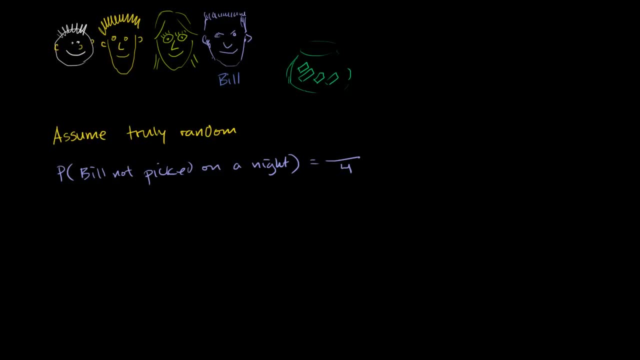 well, there's four equally likely outcomes and three of them result in Bill not getting picked. So there's a three fourths probability that Bill is not picked on a given night. Well, what's the probability that Bill's not picked three nights in a row? 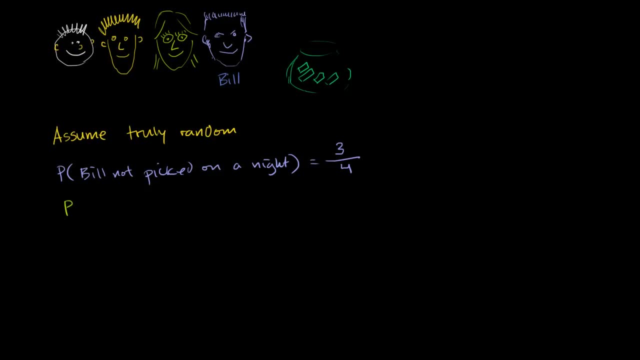 Let me write that down. So the probability Bill not picked three nights in a row. three nights in a row? well, that's the probability that he's not picked on the first night times the probability that he's not picked on the second night. 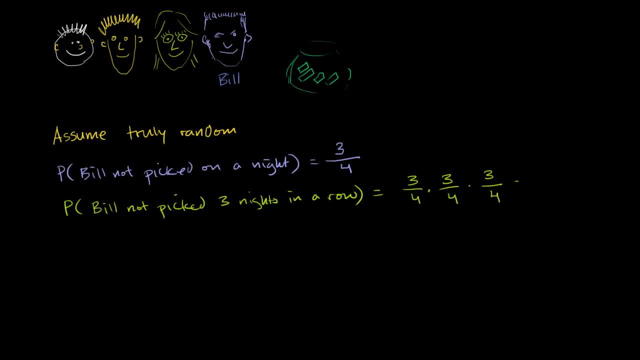 times the probability that he's not picked on the third night. So that's going to be three to the third power, or three times three times three, so that's 27,. over four to the third power. Four times four times four is 64,. 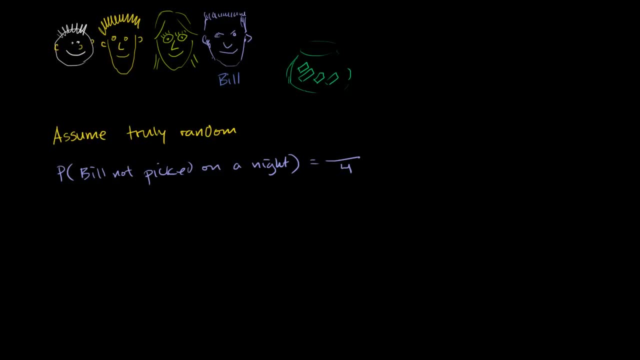 well, there's four equally likely outcomes and three of them result in Bill not getting picked. So there's a three fourths probability that Bill is not picked on a given night. Well, what's the probability that Bill's not picked three nights in a row? 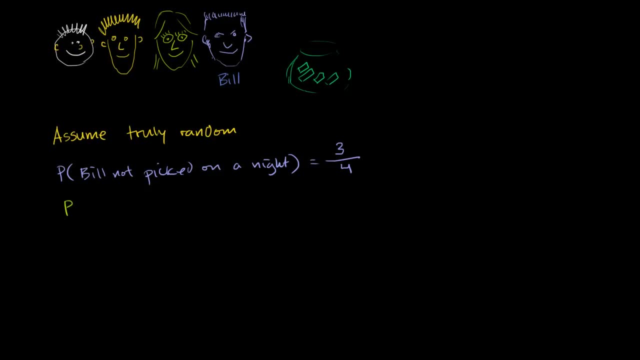 Let me write that down. So the probability Bill not picked three nights in a row. three nights in a row? well, that's the probability that he's not picked on the first night times the probability that he's not picked on the second night. 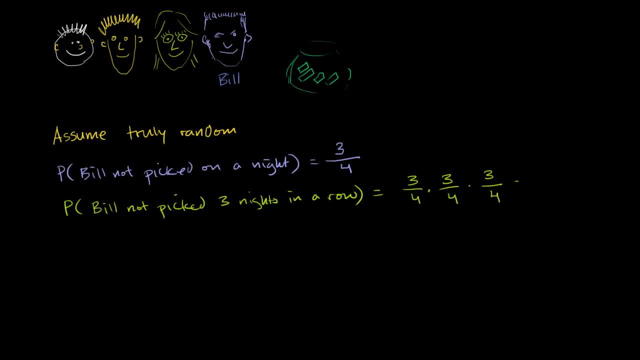 times the probability that he's not picked on the third night. So that's going to be three to the third power, or three times three times three, so that's 27,. over four to the third power. Four times four times four is 64,. 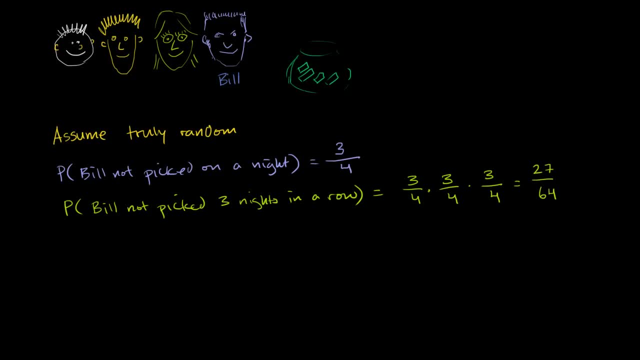 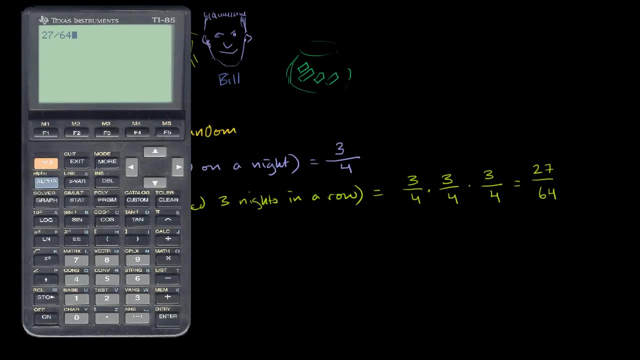 and if we want to express that as a decimal, so that is 27,. let me get my calculator out. that is 27, divided by 64, is equal to, and I'll just round to the nearest hundredth right here. 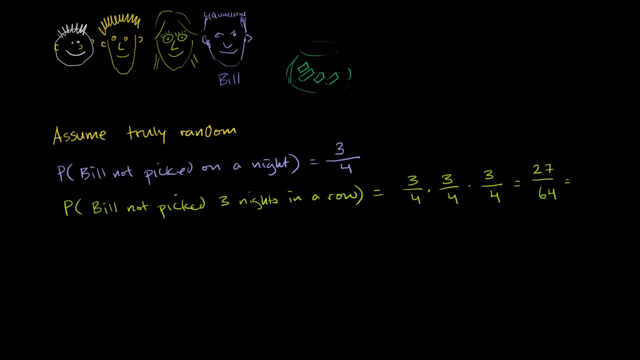 0.42.. So that is equal to 0.42.. And so this doesn't seem that unlikely. It's a little less likely than kind of even odds, but it's not. you know, you wouldn't question someone's credibility if. 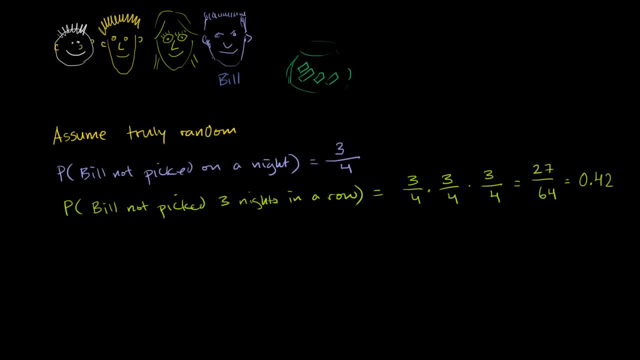 you know there's a four to the third power. you know there's a 42%- roughly a 42%- chance that three nights in a row Bill would not be picked. So this seems like, if you're assuming, truly random. 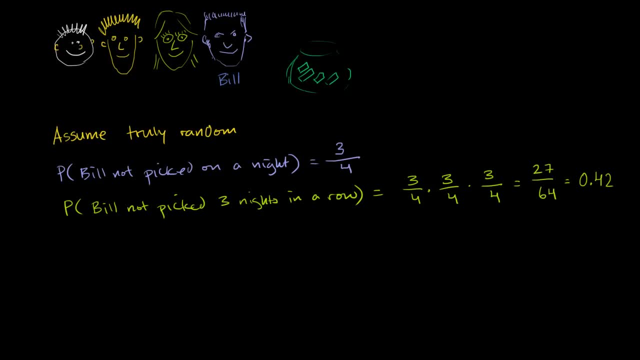 that it's a reasonable your hypothesis that it's truly random seems you know. there's a good chance that you're right. There's a 42% chance you would have the outcome you saw, if your assumption is true. But let's say 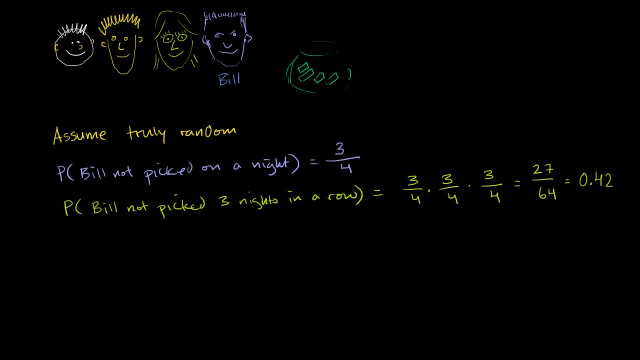 let's say you keep doing this and you trust your older brother, why would he want to cheat out his younger siblings? But let's say that Bill's not picked 12 nights in a row. So then, everyone's starting to get. everyone's starting to get a little bit. 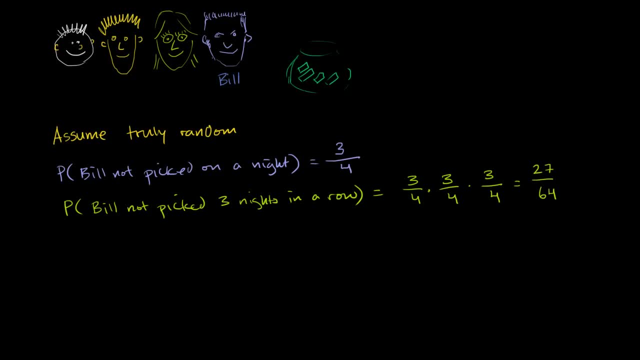 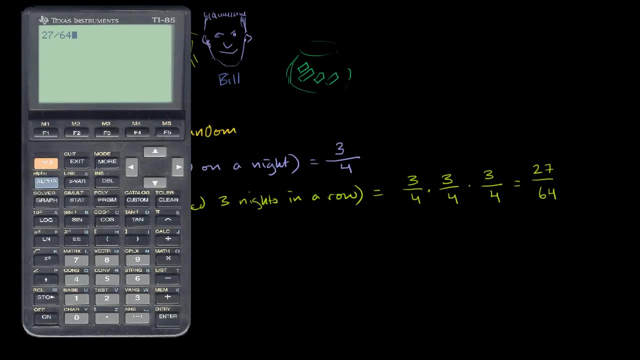 and if we want to express that as a decimal, so that is 27,. let me get my calculator out. that is 27, divided by 64, is equal to, and I'll just round to the nearest hundredth right here. 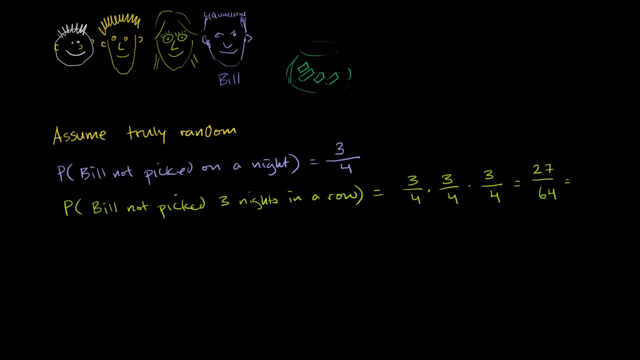 0.42.. So that is equal to 0.42.. And so this doesn't seem that unlikely. It's a little less likely than kind of even odds, but it's not. you know, you wouldn't question someone's credibility if. 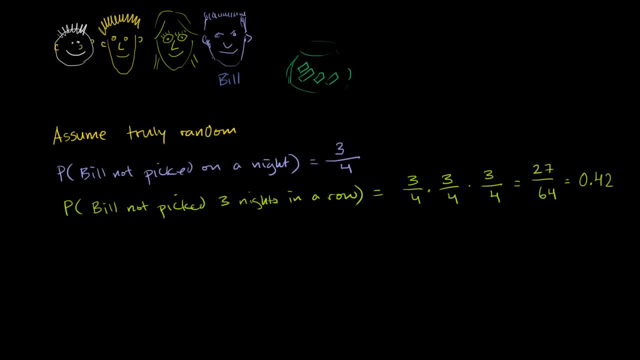 you know there's a four to the third power. you know there's a 42%- roughly a 42%- chance that three nights in a row Bill would not be picked. So this seems like, if you're assuming, truly random. 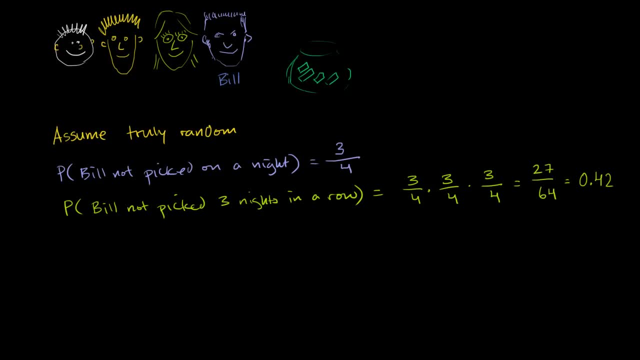 that it's a reasonable your hypothesis that it's truly random seems you know. there's a good chance that you're right. There's a 42% chance you would have the outcome you saw, if your assumption is true. But let's say 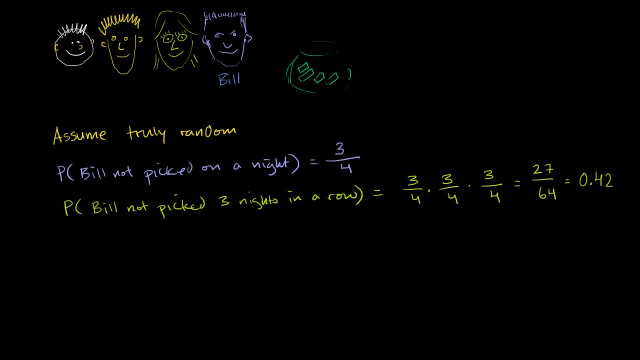 let's say you keep doing this and you trust your older brother, why would he want to cheat out his younger siblings? But let's say that Bill's not picked 12 nights in a row. So then, everyone's starting to get. everyone's starting to get a little bit. 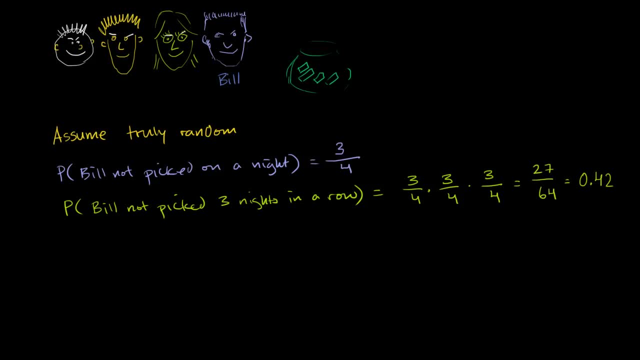 everyone's starting to get a little bit suspicious, suspicious with Bill, with Bill right over here. And so they say, well, you know, well, we're going to give him the benefit of the doubt, Assuming that he's being completely honest. 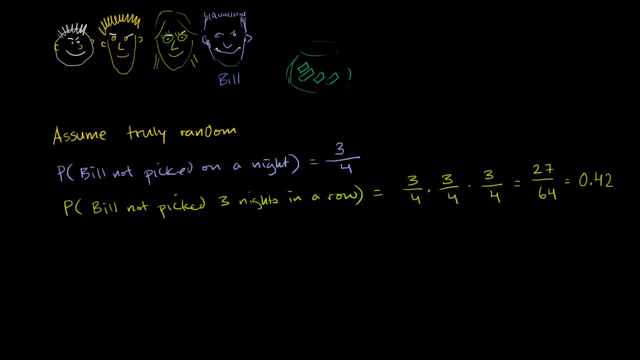 that this is a completely random process. what is the probability that he would not be picked 12 nights in a row? I'll just write that down. So the probability Bill, and it's really the same stuff that I just wrote up here. 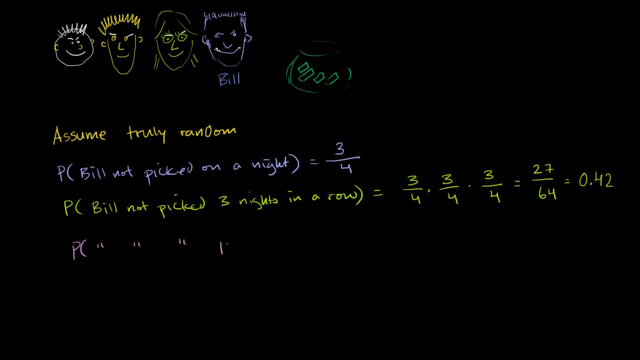 I'll just say: Bill, not picked 12 nights in a row. Well, that's going to be three. you're going to take 12 three-fourths and multiply them together. It's going to be three-fourths to the 12th power. 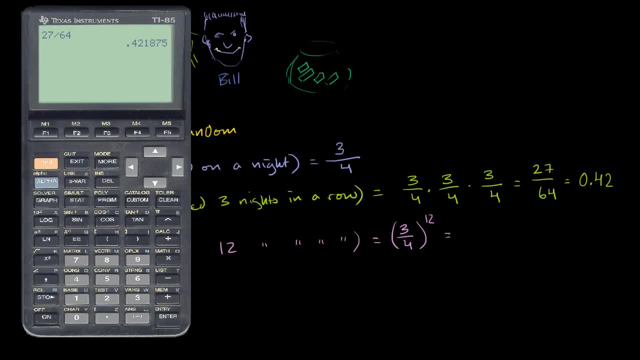 And what is this going to be equal to? Well, let's see If you take. well, three-fourths is, I'll just write three divided by three, divided by four, which is going to be 0.75,. to the 12th power. 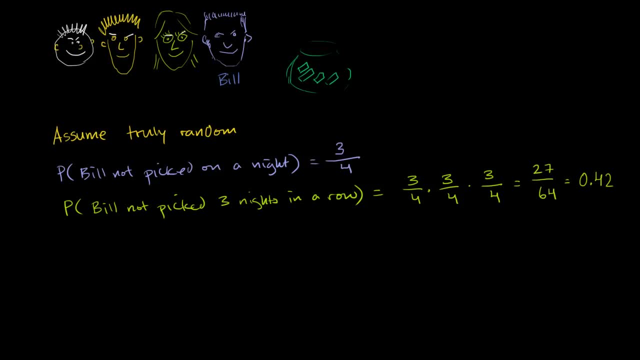 everyone's starting to get a little bit suspicious- suspicious with Bill, with Bill right over here. And so they say: well, you know, we're going to give him the benefit of the doubt, Assuming that he's being completely honest, that this is a completely random process. 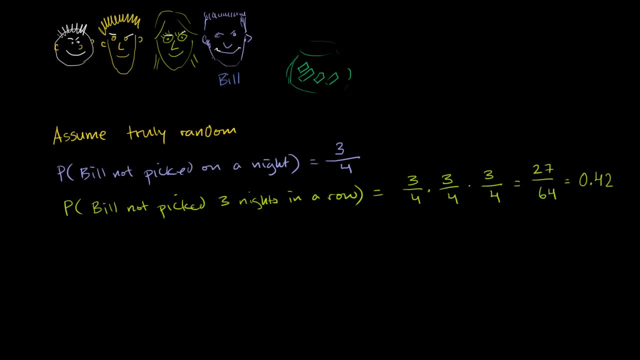 what is the probability that he would not pick 12 nights in a row? I'll just write that down. So the probability, Bill, and it's really the same stuff that I just wrote up here. I'll just say: Bill not picked 12 nights in a row. 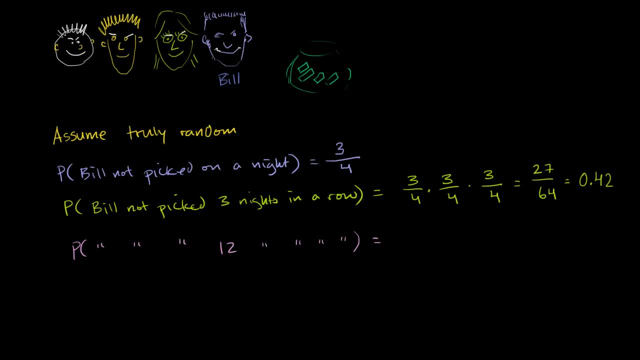 Well, that's going to be three. you're going to take 12 three-fourths and multiply them together. It's going to be three-fourths to the 12th power. And what is this going to be equal to? Well, let's see. 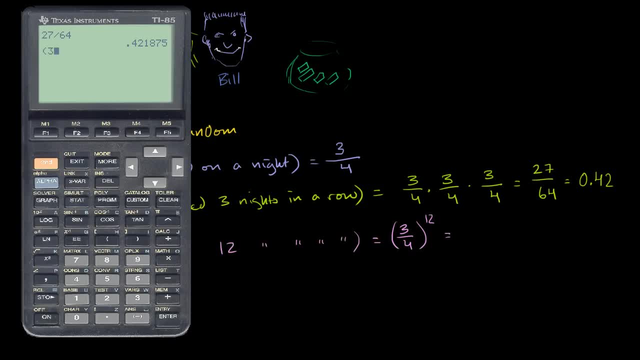 If you take well, three-fourths is, I'll just write three divided by three divided by four, which is going to be 0.75, to the 12th power. Now, this is a much smaller. this is now. 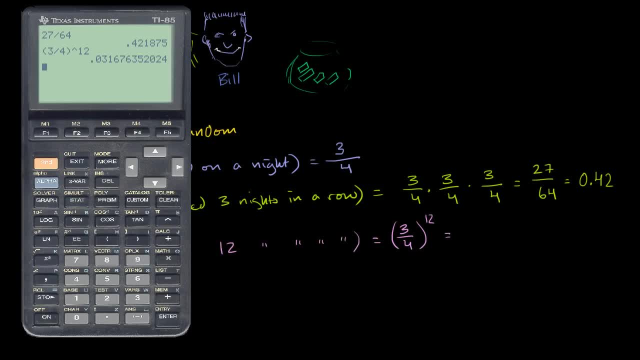 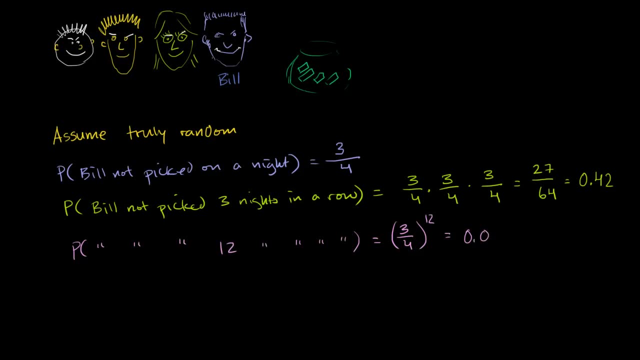 if we actually this is going to be 0.3,, I guess we could go to one more decimal place, 0.32, or we could say this is 0.032, I should say, which is equal to. 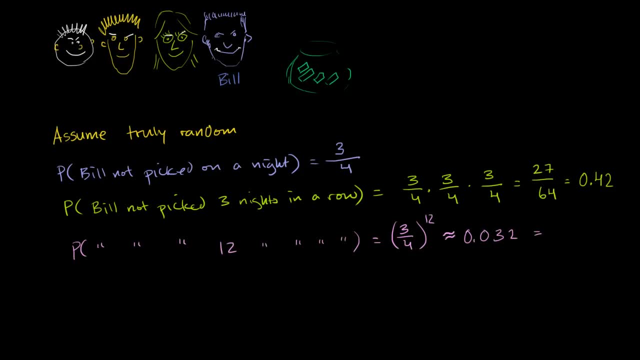 so this is approximately equal to. let me write that, which is equal to 3.2%. So now you have every right to start thinking that something is getting fishy. You could say, well, look if there was. and this is what statisticians actually do. 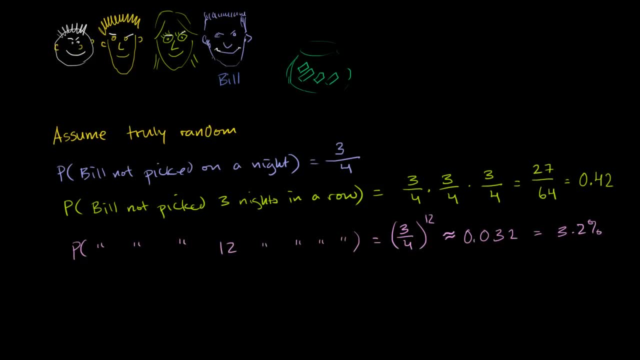 they often define a threshold. hey, you know, if the probability of this happening purely by chance is more than 5%, then I'll say, well, maybe it was happening by chance. But if the probability of this happening purely by chance was, 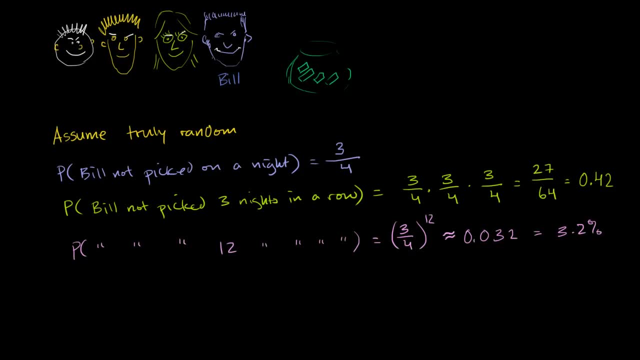 and this is the threshold that statisticians often use. it is 5%, but that's somewhat arbitrarily defined. But this is a fairly low probability that it would happen fairly by chance. So you might be tempted to reject the hypothesis. to reject the hypothesis. 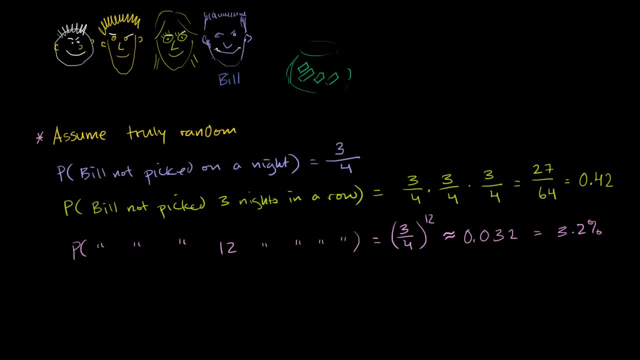 that it was truly random that Bill is cheating in some way, And you could imagine if it wasn't 12 in a row, if it was 20 in a row, then this probability becomes really, really, really, really, really small.